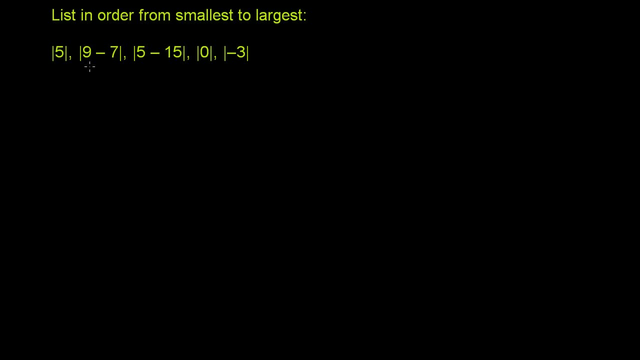 inside of the absolute value sign, it becomes positive. If it's already positive, it stays positive. So let's think about these numbers. So the first one is the absolute value of 5.. How far is 5 away from 0?? 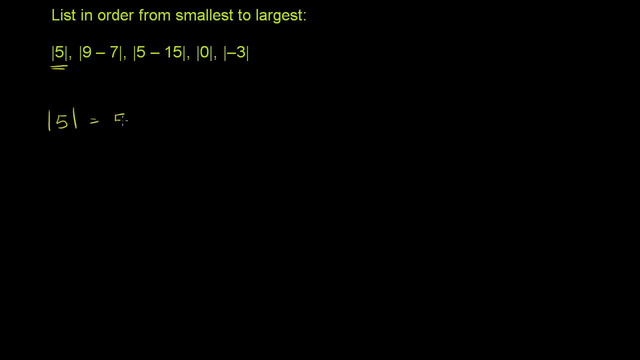 Well, it's 5 away from 0. So it's equal to 5.. So if I were to actually draw a number line, you would see that 0 is here, 5 is over here, This distance, right there is 5.. 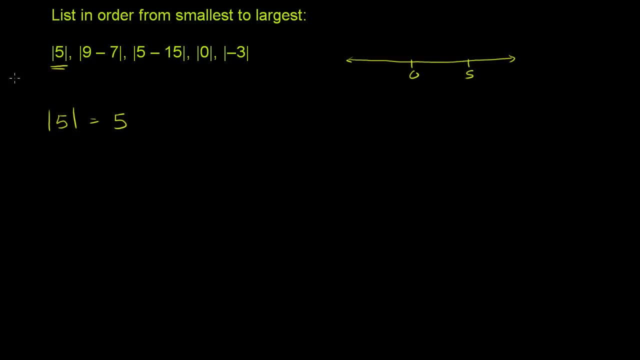 So the absolute value of 5 is 5.. Now, the next quantity they want us to figure out is the absolute value of 9 minus 7.. Well, this is the same thing as the absolute value of 2, 9 minus 7.. 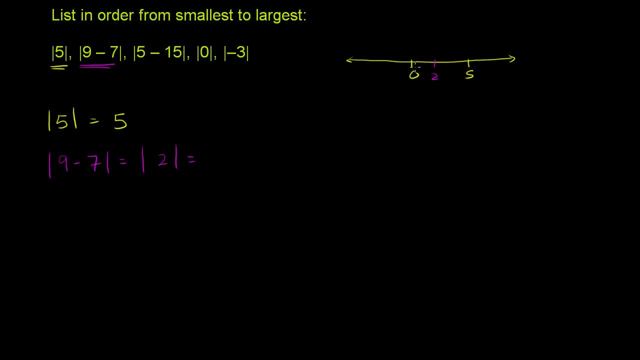 9 minus 7 is 2.. And once again, 2 is just 2 units away from 0. So it's just 2.. If you have a positive value in the absolute value sign, it just is itself. The absolute value of 2 is 2.. 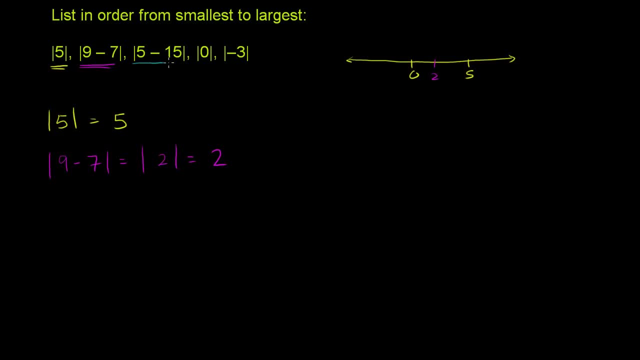 Then we have the absolute value of 5 minus 15.. Well, that's going to be the same thing as the absolute value. 5 minus 15 is negative 10.. So it's the same thing as the absolute value of negative 10.. 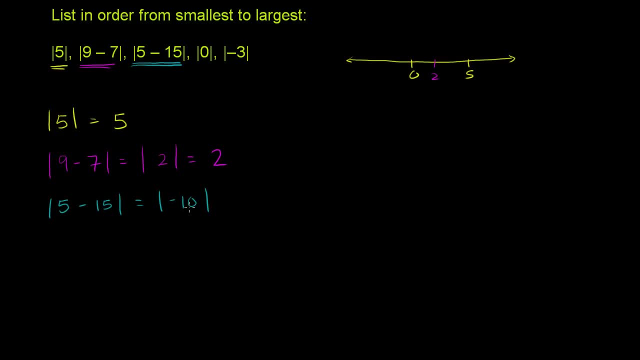 Now there's two ways you can think about it. If it's a negative number inside of the absolute value sign, it just becomes the positive version of it, So it just becomes 10.. Another way to think about it is if you had negative 10, you 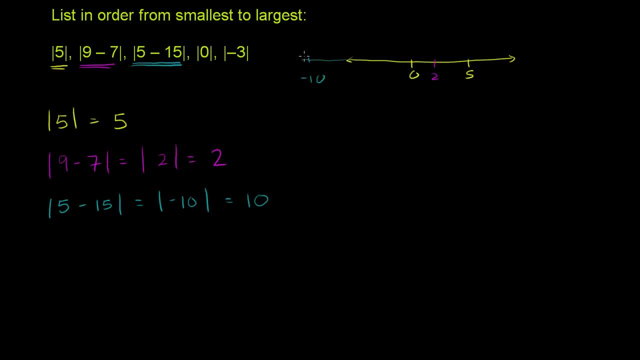 would plot it, it would be out here someplace: Negative 10, we'd have to extend the number line- It is 10 to the left of 0. That's what the absolute value is telling us. Then we have the absolute value of 0.. 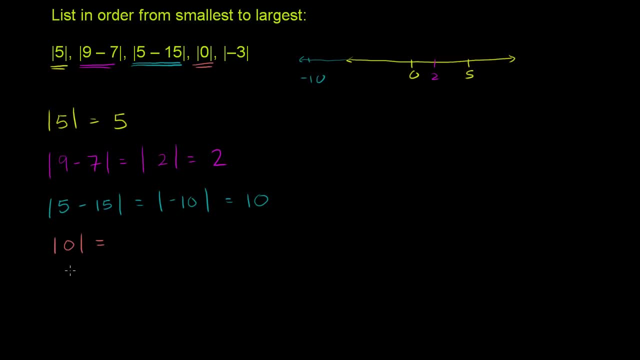 We have the absolute value of 0. Well, 0 is just 0. away from the number line, The absolute value of 0 is just 0. That is just 0. That's just right there. It has no distance from the origin. 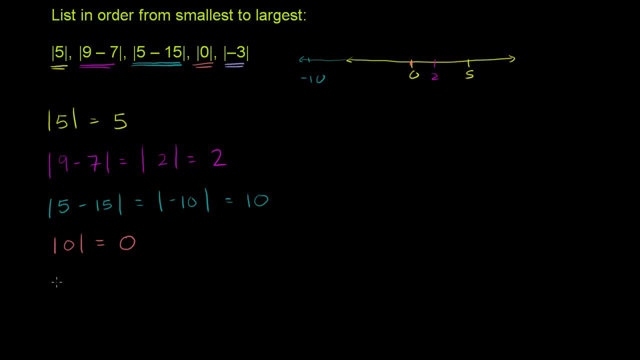 And then, finally, we have the absolute value of negative 3.. That's 3 to the left of 0, or you can just think of it as getting rid of this negative sign, So it is equal to 3.. So now that we've expressed them all as just simple,